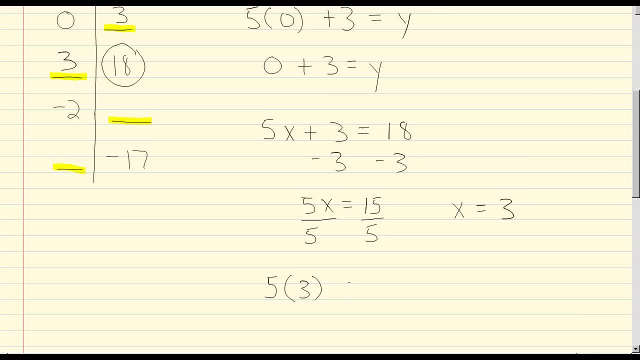 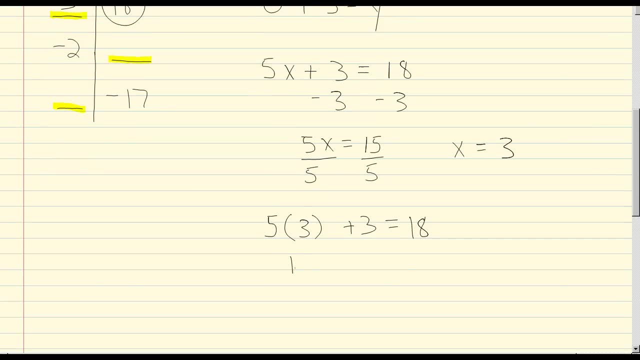 So you go: 5 times 3, plug in a 3 for the x plus 3 equals 18.. So we're going to see if that's true, 5 times 3 is 15, and then 15 plus 3 does equal 18,. 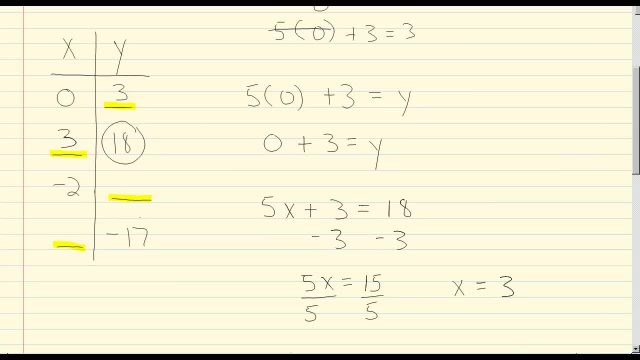 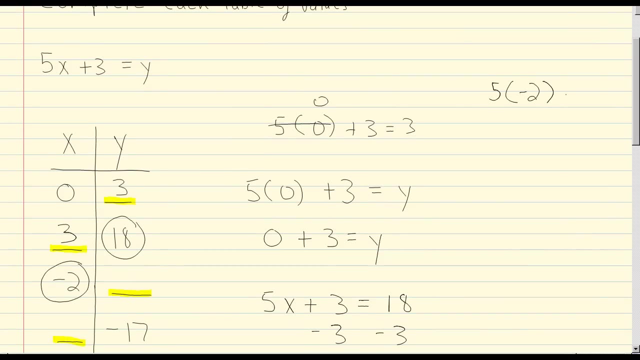 so that is a true statement. Let's look at our next value to be completed. We're given a negative 2 for the x and we want to find the y, so let's come up here. So we know that x is negative 2, so we're going to have 5 times negative 2 plus 3 equals. 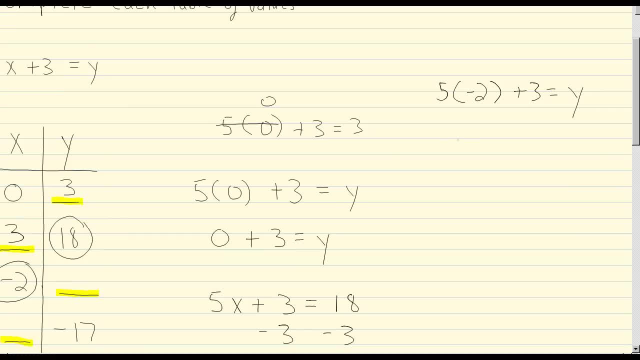 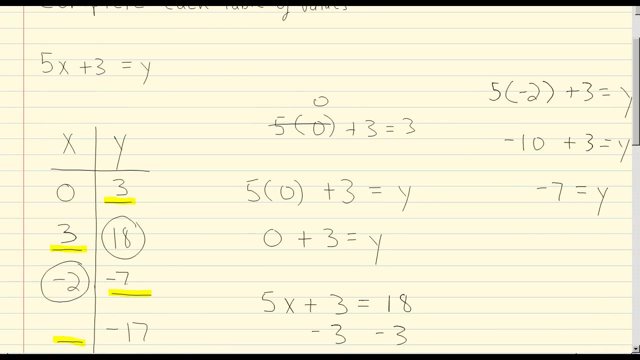 y 5 times negative. 2 would be negative 10, then plus 3 equals y and so negative 10 plus 3 is negative 7, so y is going to be equal to negative 7.. You come over here and just plug in a negative 7, and if you want to check that you're going. 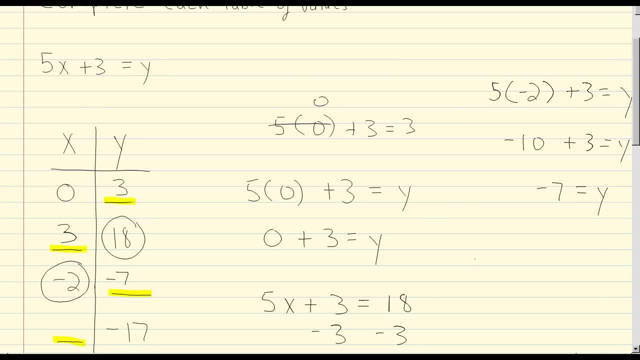 to plug in a negative 2 for x and a negative 7 for y, So you'd have 5 times negative 2 plus 3, and that should be equal to negative 7.. 5 times negative 2 plus 3 equals y. 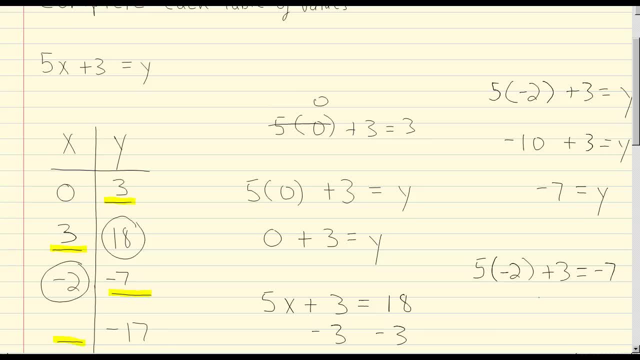 5 times negative. 2 is negative 10, negative 10 plus 3 is negative 7, so you can see that this would be negative 7 equals negative 7.. That's, of course, a true statement, so we know that's correct. 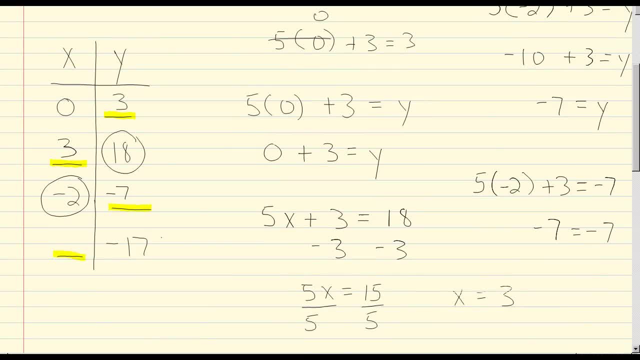 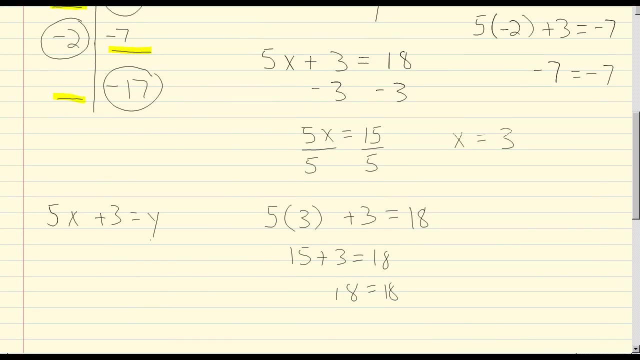 All right, let's look at our last value to be filled in. We're told that y equals negative 17,. so we want to find x. So our equation was: 5x plus 3 equals y. so we're going to plug in a negative 17 for y. 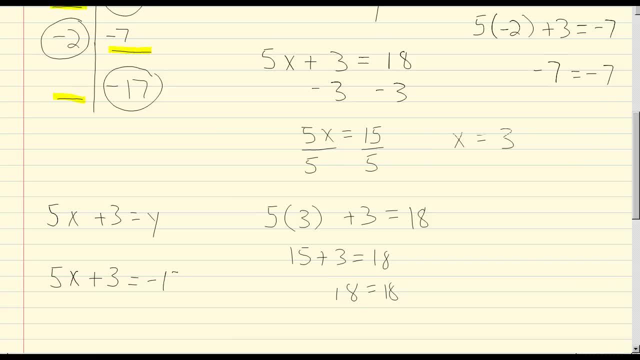 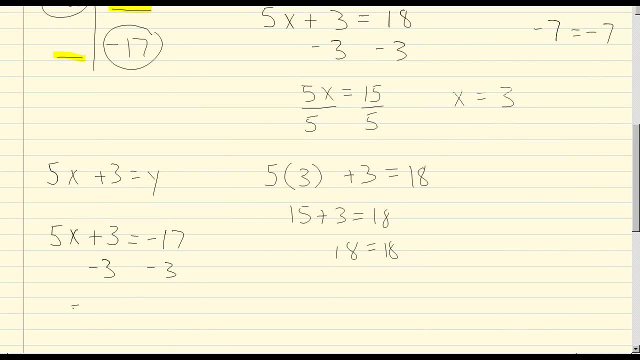 so we'll have: 5x plus 3 equals y, 5x plus 3 equals negative 17,. and of course we want to start out by subtracting 3 from both sides of this equation. so we'll have: 5x is equal to negative 20, and now we want. 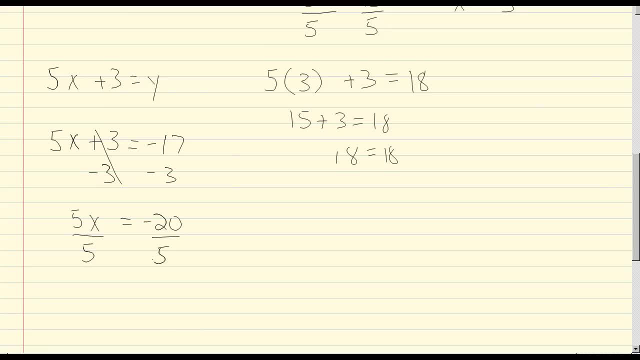 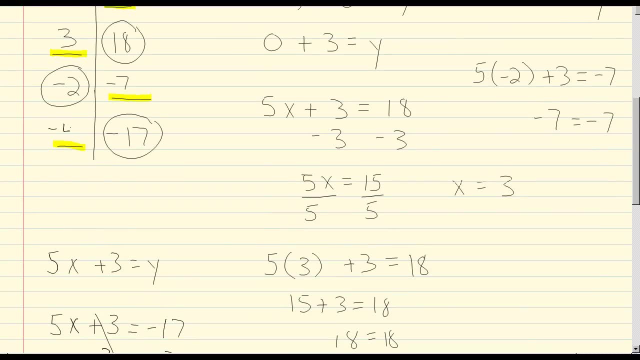 to divide both sides of the equation by 5, and we're going to get, x is equal to negative 4.. So we'll go back up here and plug in a negative 4, and if we want to check this, we're going. 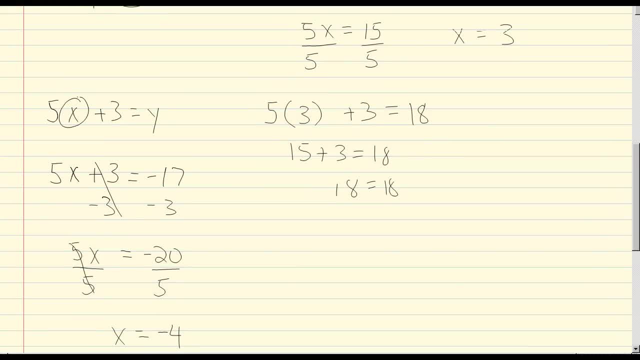 to plug in a negative 4.. So we're going to plug in a negative 4.. We're going to plug in a negative 4.. A negative 4 for x and a negative 17 for y, so you have 5 times negative 4 plus 3 equals.